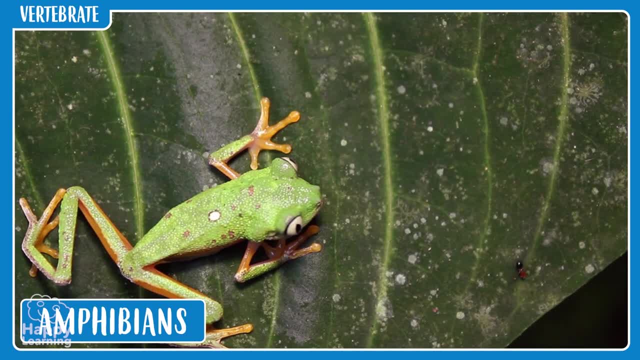 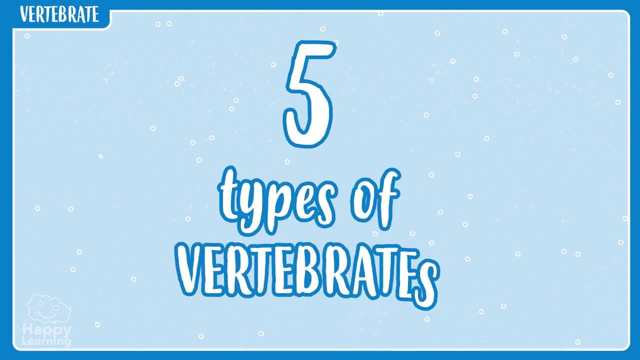 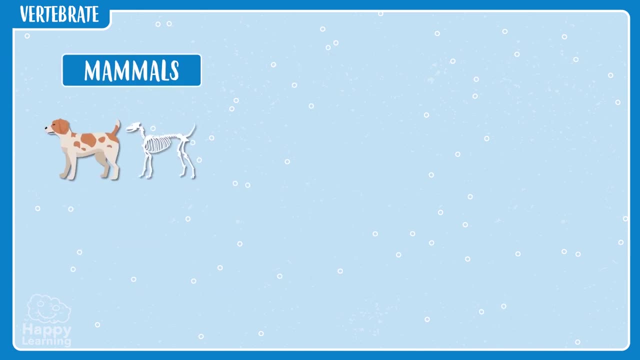 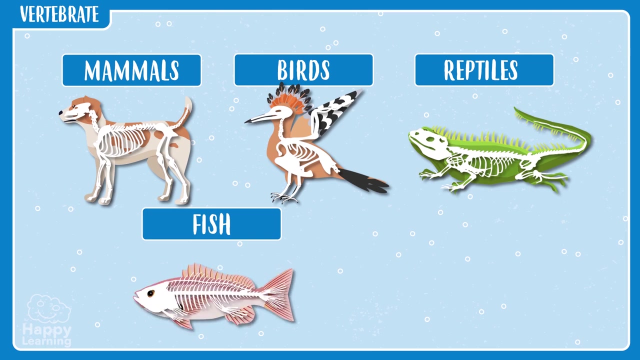 And amphibians, like this little jumping frog. Remember, there are five types of animals that have bones. There are five types of vertebrates: Mammals, Birds, Reptiles, Fish And amphibians Within the group of invertebrates. 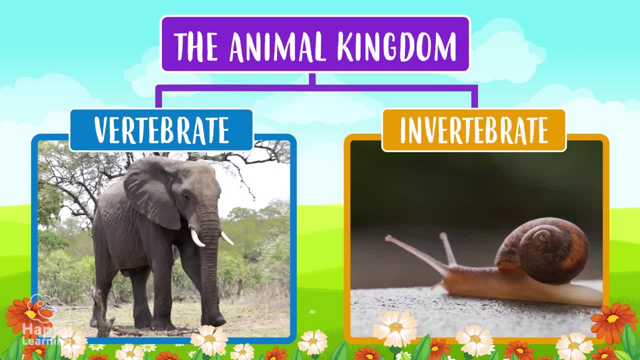 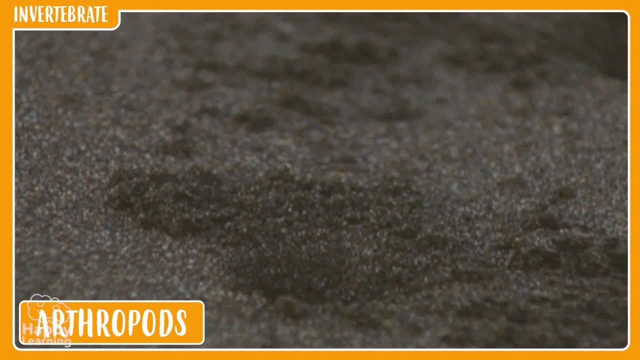 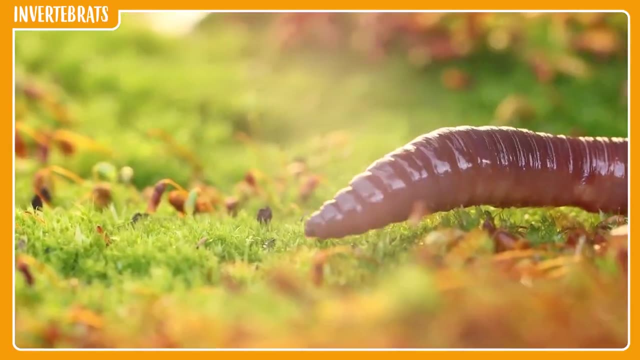 In other words, those animals that don't have bone. There are arthropods Like this shy crab, Mollusks Like this octopus and its eight tentacles, Anelids Like this worm Echinoderms. 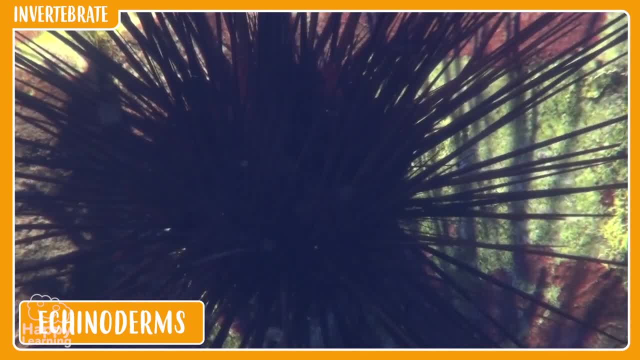 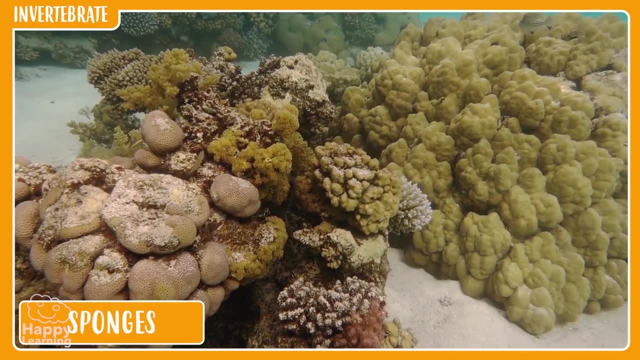 Like this spiky sea urchin, Sponges And Nadarians, Like this shiny jellyfish. They really do have some strange names: Arthropods, Mollusks, Anelids And Mammals. 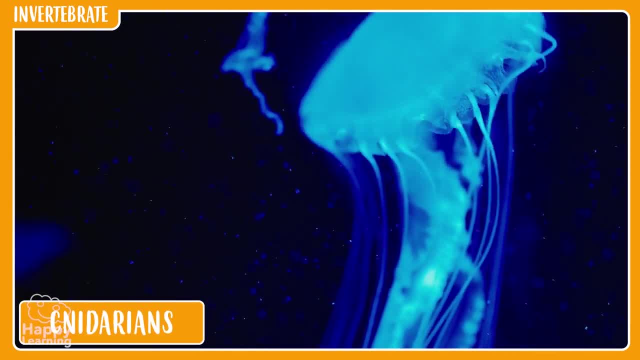 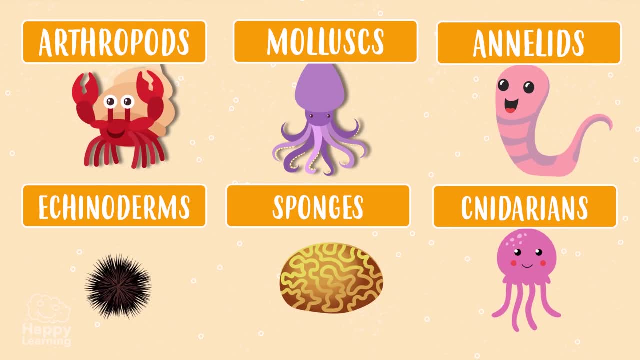 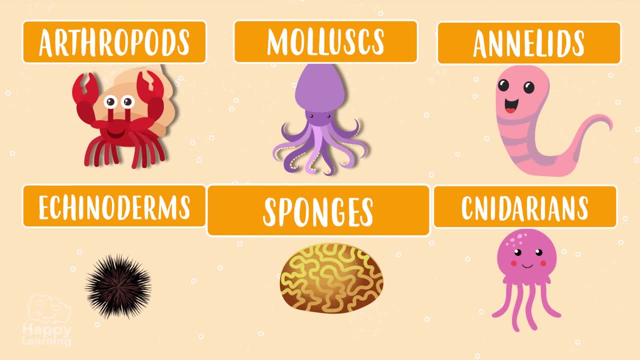 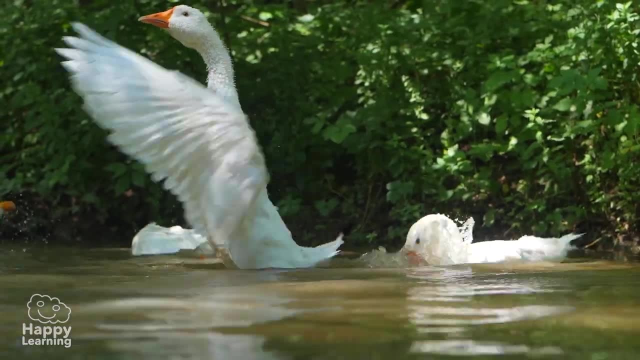 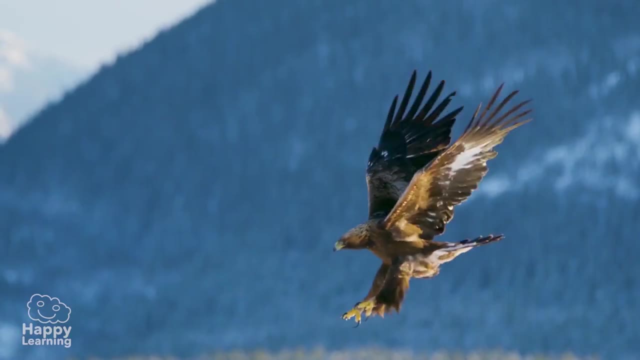 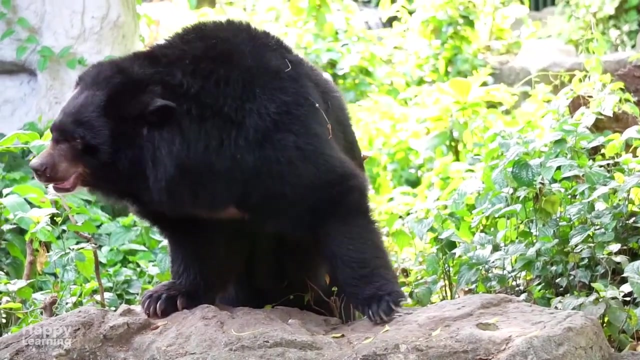 And Sponges, And Sponges And Nadarians. They really are very curious, aren't they? Now let's see if we can distinguish which animals are vertebrates and which are invertebrates. Is this dancing bear a vertebrate or invertebrate? 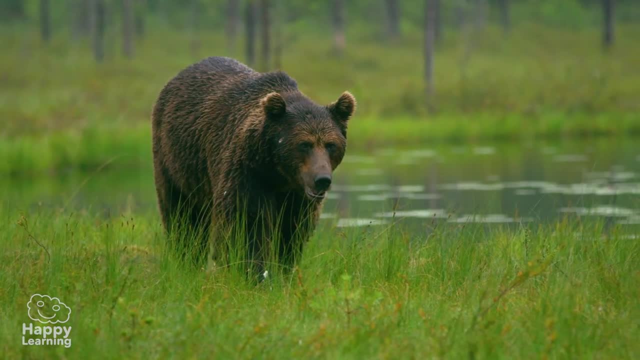 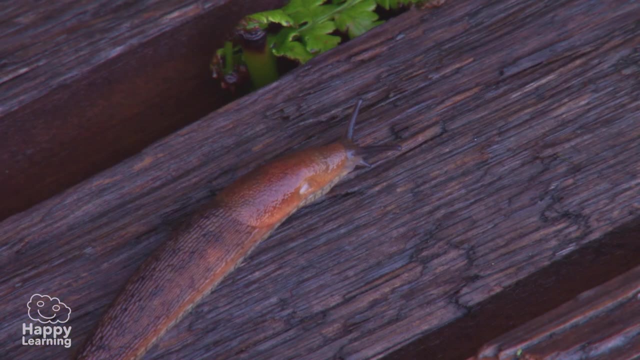 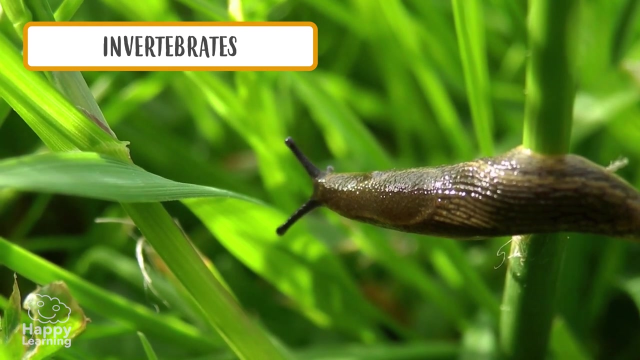 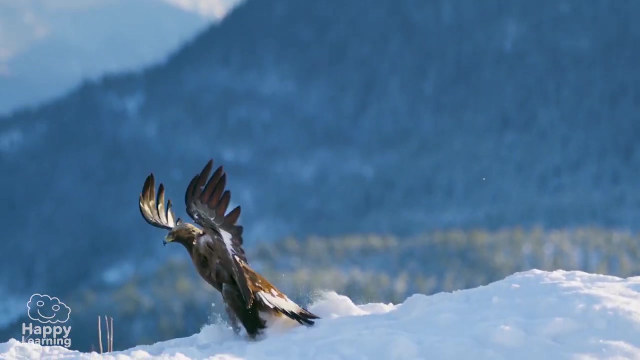 Of course, Bears are vertebrate animals, They have bones and they are also mammals. What about this slug? Slugs are invertebrate animals, They are mollusks, They have no bones and are very soft, And this eagle Eagles do have bones. 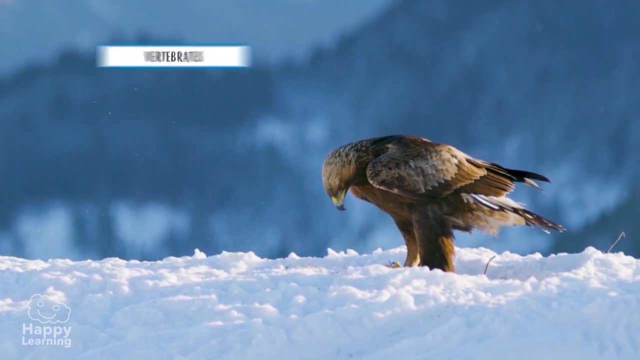 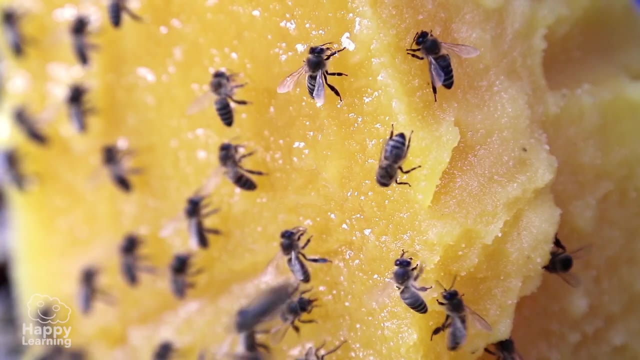 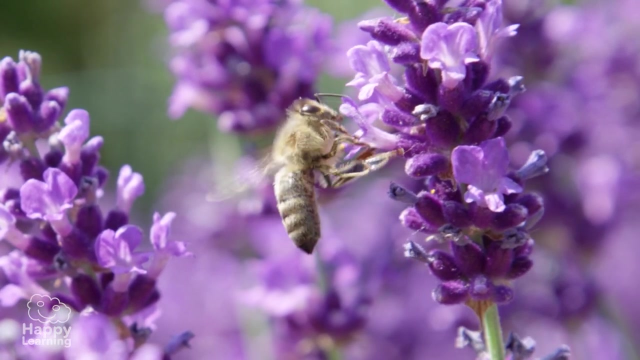 They are vertebrates, They are birds, they're animals, vertebrate animals. And finally, these bees. hmm, are they vertebrates or invertebrates? Bees do not have an internal skeleton and they do not have bones. They are arthropods, in other words.